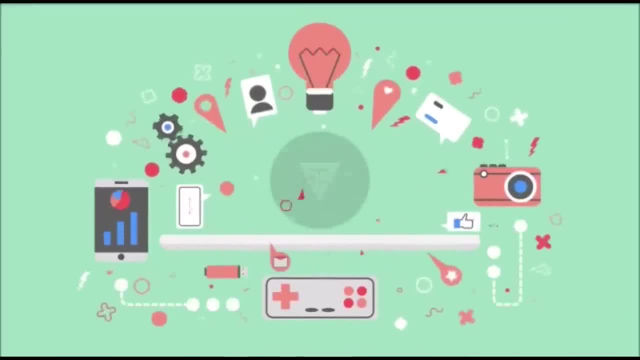 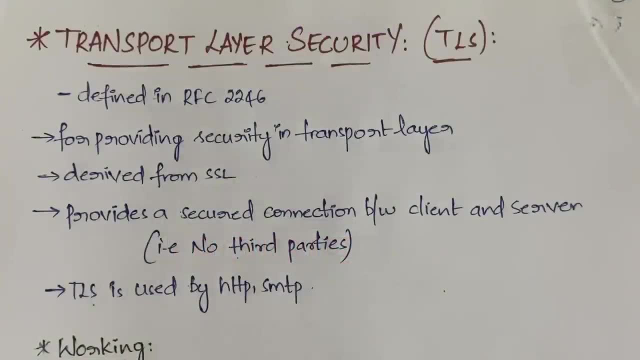 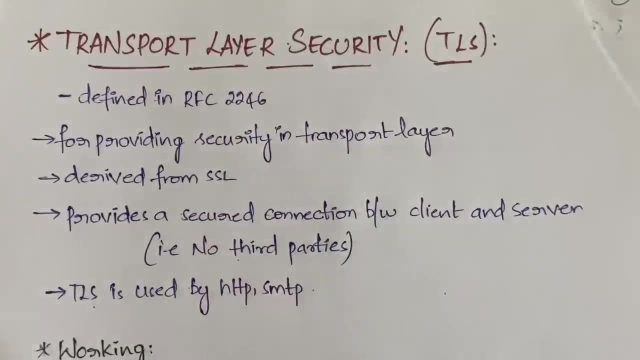 Hello everyone, welcome back to my YouTube channel, TrebleFree. In this video, I am going to explain you about the transport layer security, which is, in short, also called as TLS. So, basically, this is also a very short video and a very easy video, like the previous one, like the. 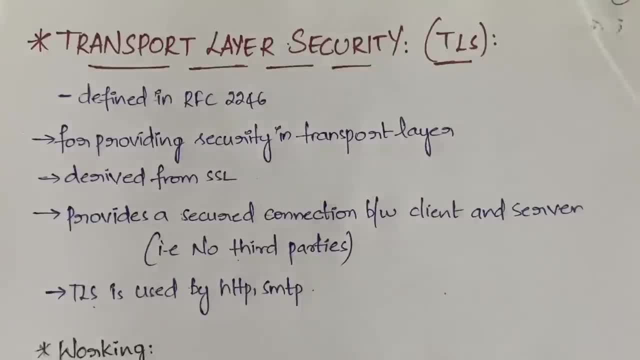 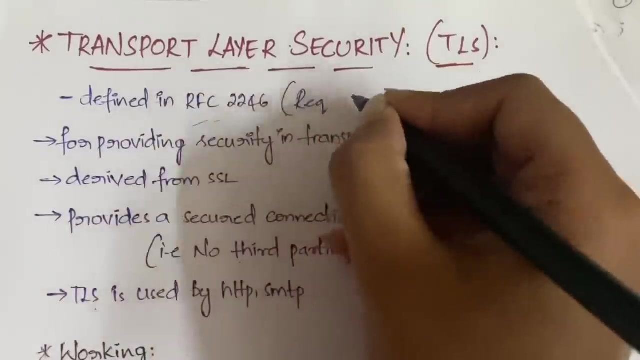 previous one, which we have discussed: HTTPS protocol video. So the same. this is also very simple, very short and very easy, So let us get into the video. First of all, it is defined in RFC 2246.. What do you mean by RFC? It is request for comments. Request for. 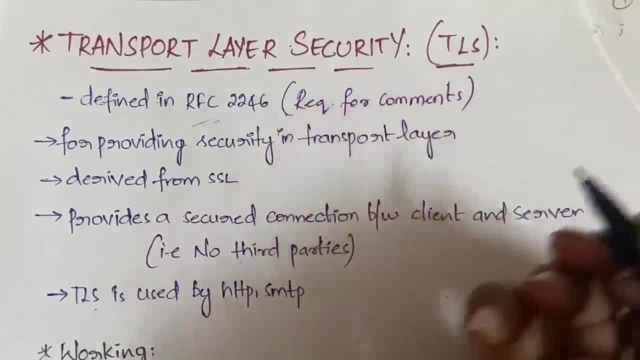 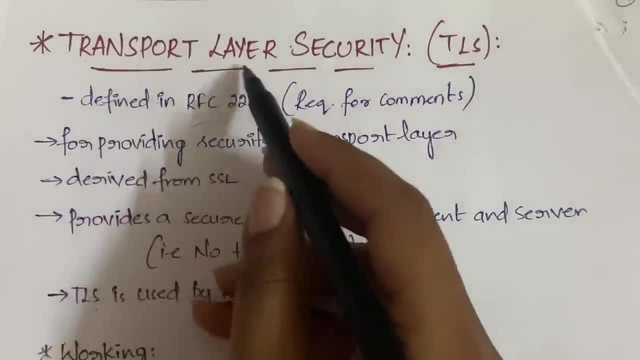 comments. Okay, so it is defined in RFC 2246.. And next, why we need this TLS: transport layer security. Transport layer security is needed for transport layer security. So it is needed for transport layer security. So it is needed for transport layer security. Transport layer security is needed for transport layer security. 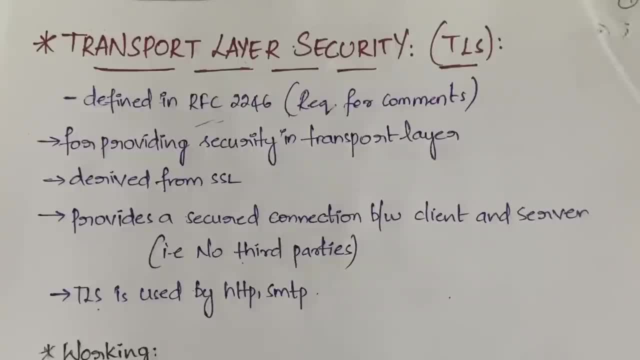 So it is needed for transport layer security. So it is needed for transport layer security. So when the data is traveling from transport layer to its next layer or to its below layer, we need to provide the security to the data right, So the data should not be lost. So 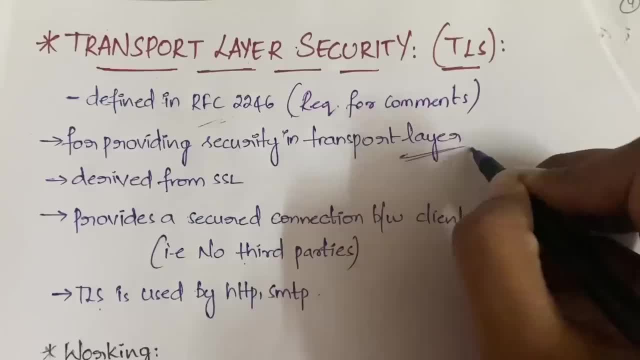 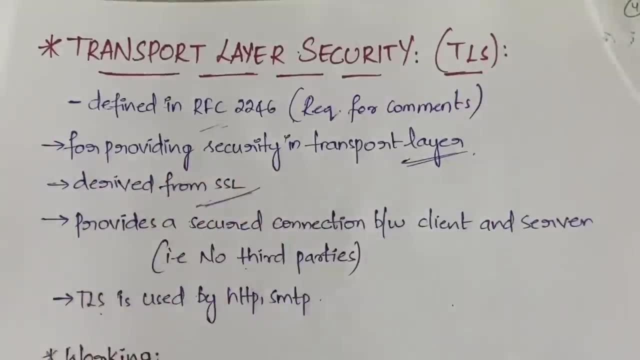 in order to provide that security, we will be using this TLS- got it- Transport layer security. It is used for providing the security in the transport layer got it And it is derived from SSL. Derived from SSL in the sense we will be using some concepts, which 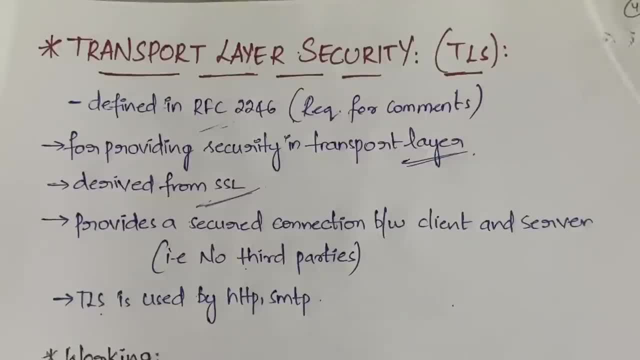 are related to SSL here. that is the handshake protocol. I have already explained about SSL handshake protocol. If you have any questions, feel free to ask me in the comments section. If you have missed that video, just go back to that video and first learn that and then 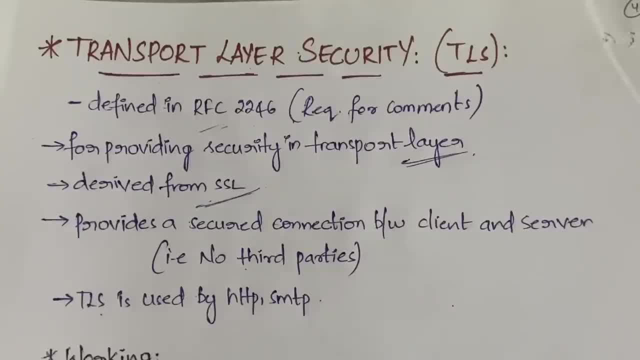 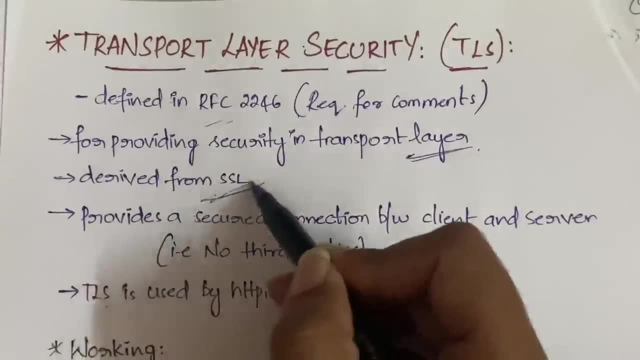 come here. So it completely the working of this transport layer security completely depends on the SSL handshake protocol itself got it Now, so done. derived from SSL is done. It provides a secured connection between the client and the server so that no third party. 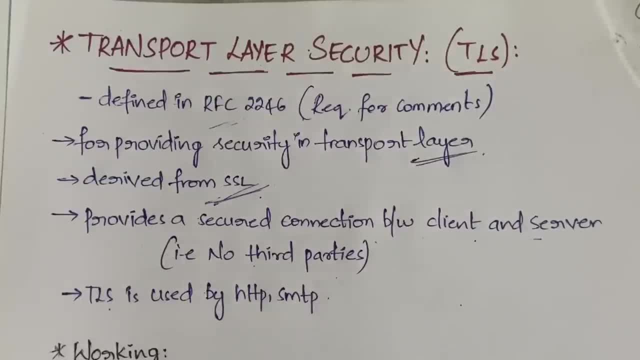 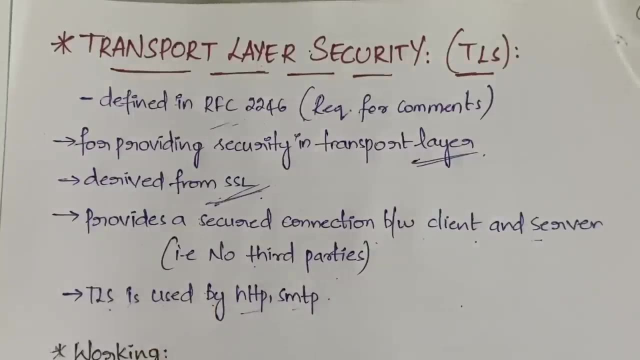 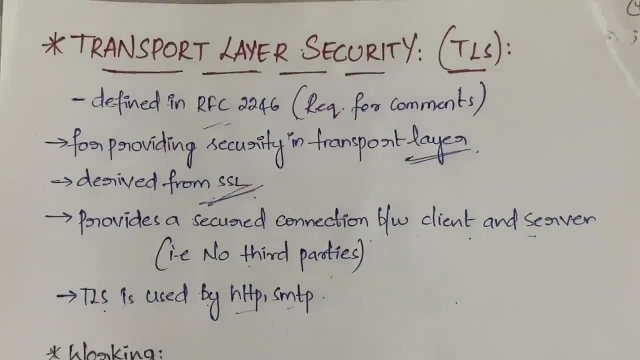 can interfere in between. No hacker or no attacker can come in between and steal the data right. So this is about the security, that is, the security between the client and the server. got it? The security said isup schemes. The next video is about TPPA. 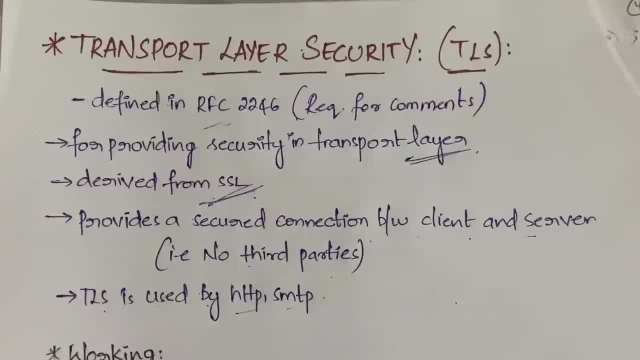 As you can see, the command is used by fingersettab. As we have seen here before, it provides security derived from the ssls, um and secure socket layer protocol, and also it is mainly used for providing the connection between the client and the server, so that the data is not lost or data is not. 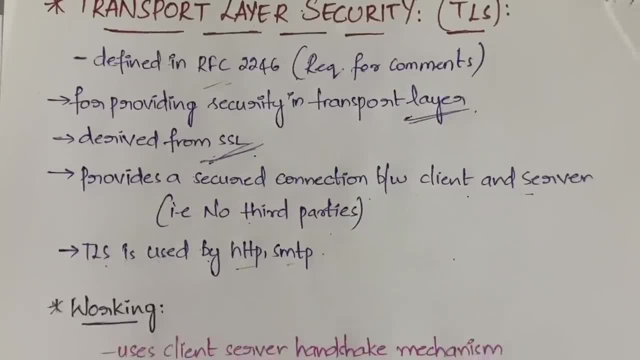 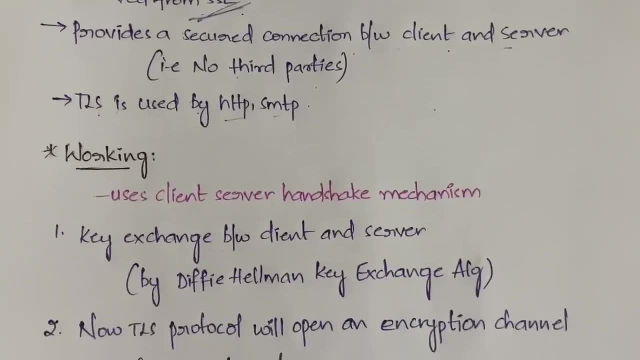 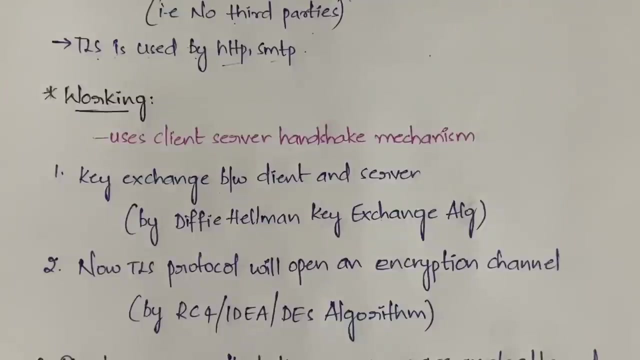 attacked by the third party got it and it is used in many of the mail transfer, message transfer, file transfer protocols now working. so, as i said, it uses the handshake mechanism right in ssl. we have already learned about what handshake mechanism is, so here it uses the client server handshake. 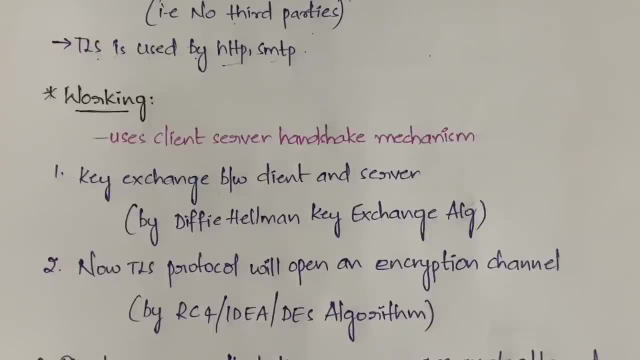 mechanism, that is, the handshake will happen between the client and so. so that is the main concept here. got it first. what happens is in handshake mechanism, first what we will be doing. we will be establishing a connection with the server, right. so here also, first we will be. 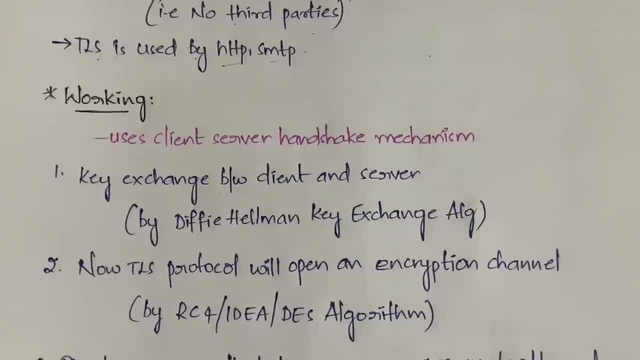 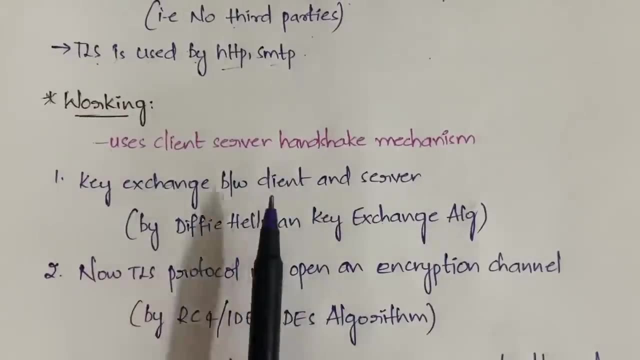 establishing the connection between the client and server. it can be a wireless connection, it can be a wired connection or it can be anything right. so first what you have to do is you need to establish the connection. once you do the establishment of the connection, here exchange will happen between the client and server. client and server will exchange their 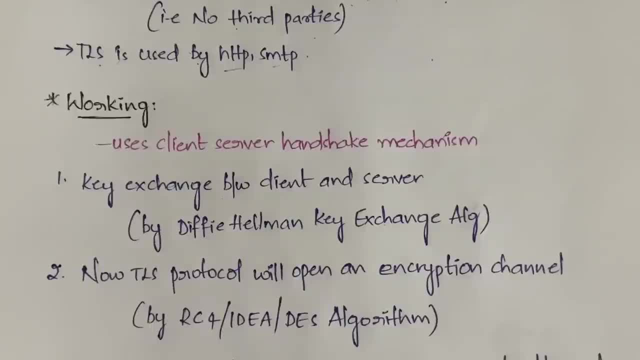 keys and they will cross check whether this is an appropriate client or not, and this client also will check whether this is an appropriate server or not. right first, key exchange will happen. now that key exchange may happen through dph helman key exchange algorithm, i already explained. 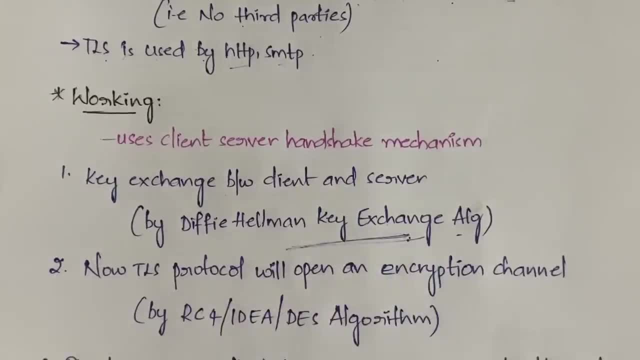 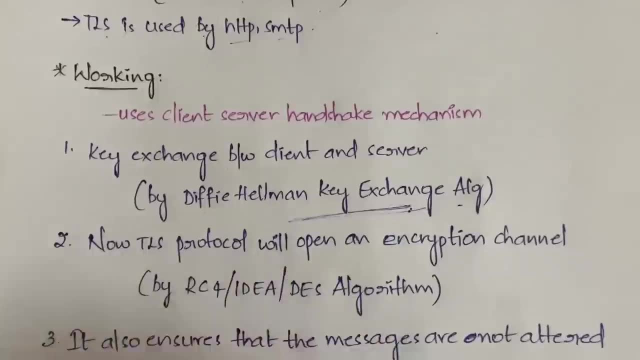 about this dph helman key exchange algorithm in my previous videos. so now the second. so once key exchange is successful in the second step, what happens is tls protocol will open an encryption channel. why encryption channel? in order to do the encryption of the data right. so if the server has 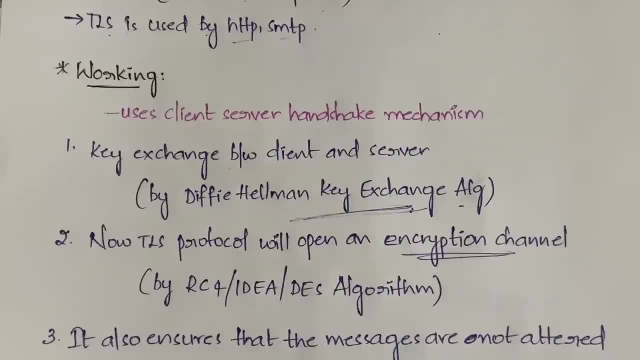 to send some data to client, or if the client has to send some data to the server, it will not just like that. it will not send, right. so it will have to encrypt the message in order to make the message as a ciphertext so that nobody can understand, right? so here also now tls protocol will open. 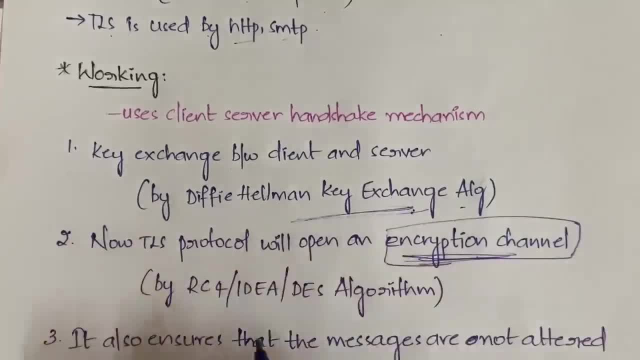 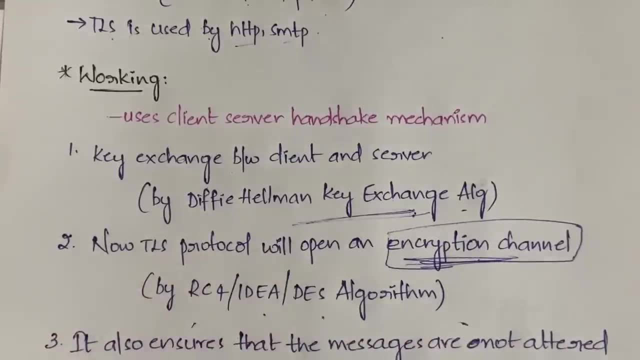 an encryption channel where encryption is performed and this encryption can be done by rc4 algorithm or idea algorithm or des algorithm or aes algorithm algorithm. so whatever encryption algorithms you are having, you can apply or any of the algorithm according to the type of the data you have, and you can do the encryption in the encryption channel. 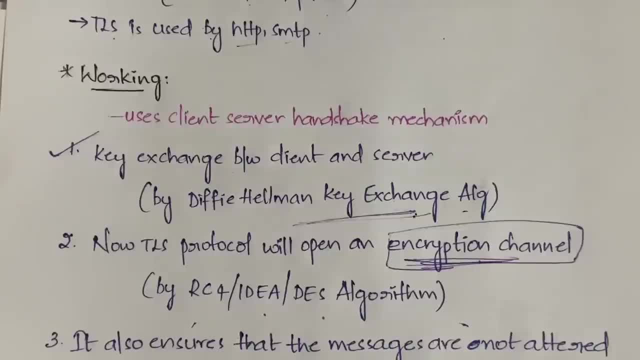 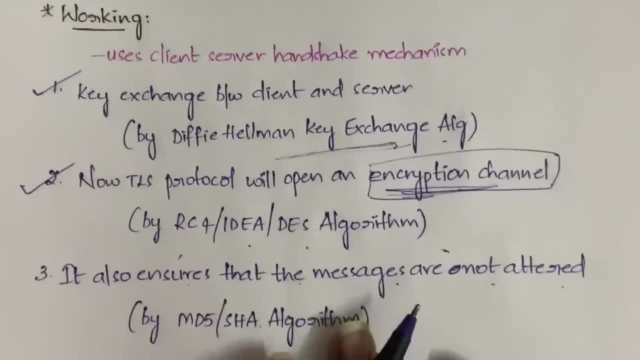 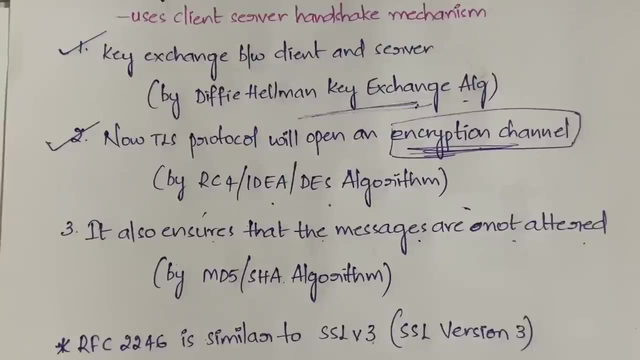 done so. first step, that is, key exchange between client and server is done, and in the second step, encryption is also done. set now in the third step. it also ensures that the messages are not altered. so, uh, this tls protocol. it will not only see that there, uh. so yeah, wait um tls protocol. 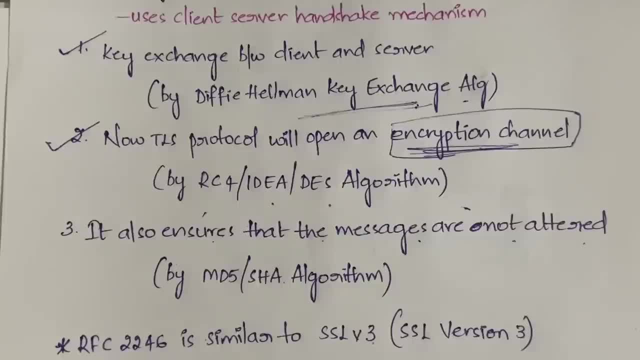 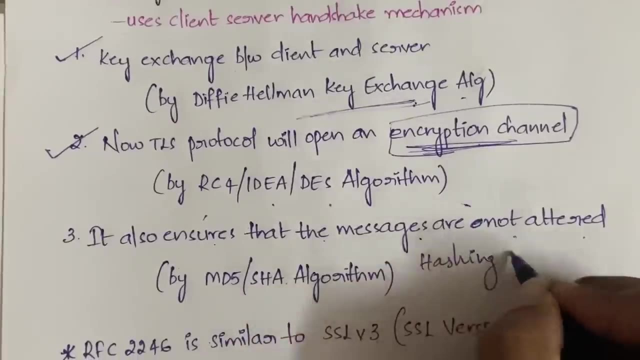 only ensures that there is no attacker in the network and but also it ensures that the messages are not altered. the messages are not changed. okay, so it ha. it is done by any of the hashing algorithms. so this um can be done by any of the hashing algorithms and like md5 or sha algorithm. 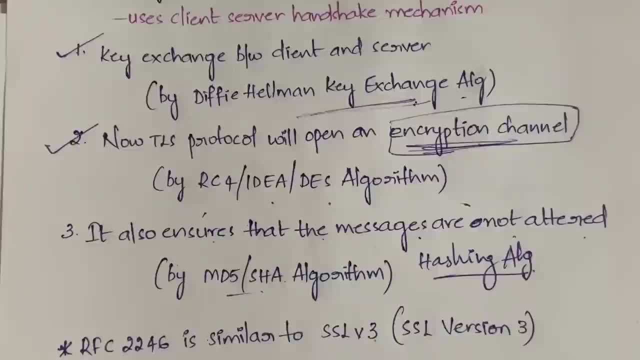 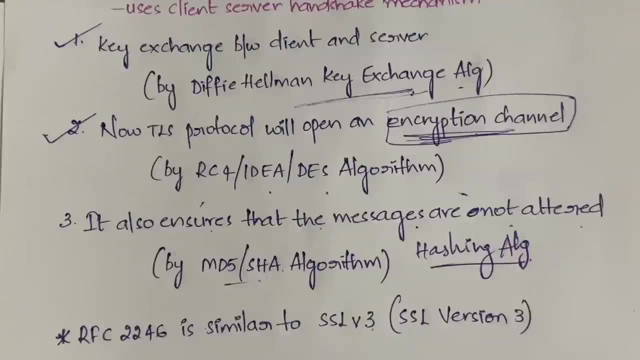 got it. so i hope you guys are clear what happens in this uh tls. it is very simple. uh, first a connection is established between the client and the server. then the client and server both will exchange their keys with each other to check the authorization and then, after checking, it will. 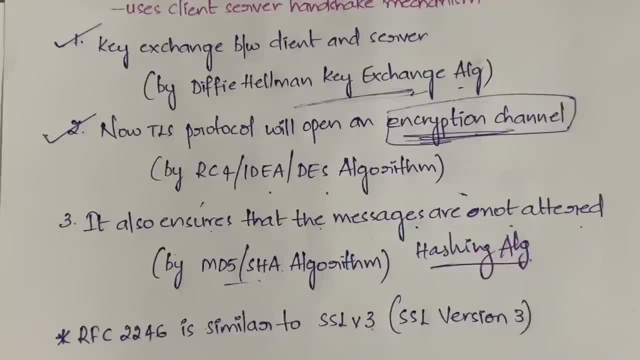 now, if, if tls thinks that, if the server thinks that, okay, this client is an appropriate client so i can share my data with him, then the tls protocol will open a encryption channel where the encryption of data will happen later. tls protocol will also ensure that the data which 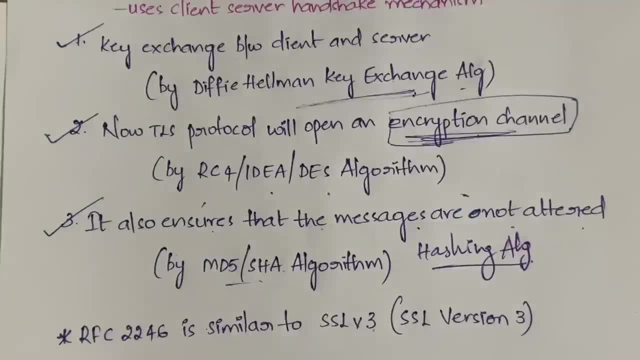 is being sent from the client to the server or server to the client is not changed in between. got it by the help of some hashing algorithms like sha or md5. so this is about the uh tls protocol and also rfc. that is a request for comments. double to four: six. i said right it.